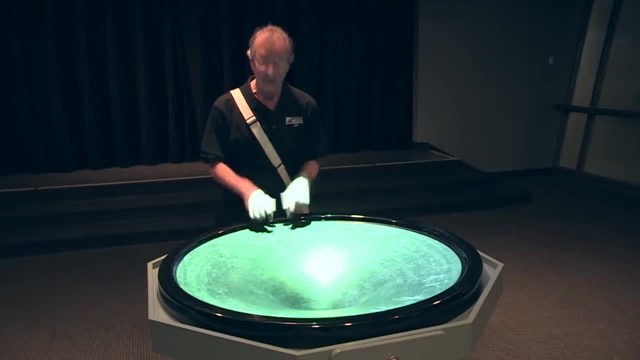 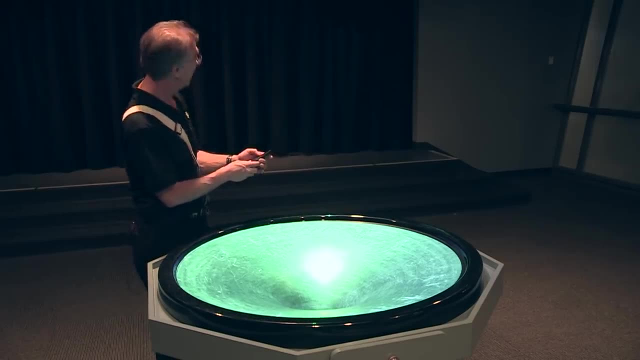 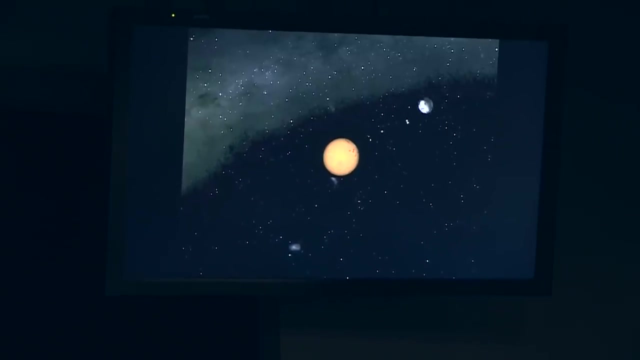 Hi, my name is Eddie, and I'd like to show you a little bit of a demonstration about gravity. So first off, let me show you what I am talking about. There is a picture of the Earth going around the sun, And people have known for a long time that the Earth goes around the sun, but they didn't know why that was, And so what I'm going to try to do right now is create that same image, two different ways of 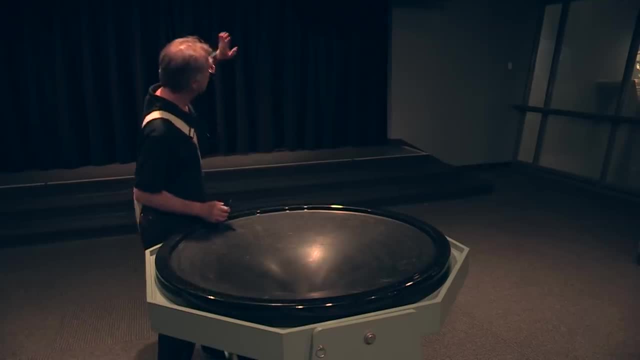 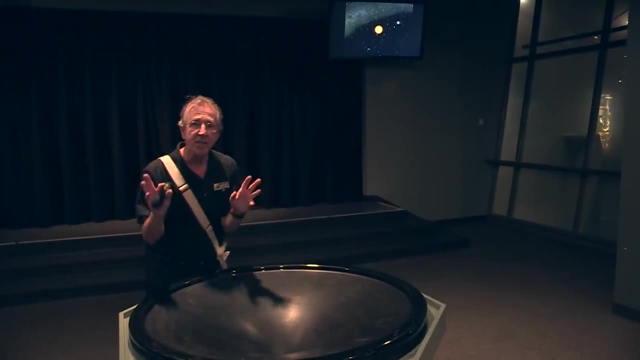 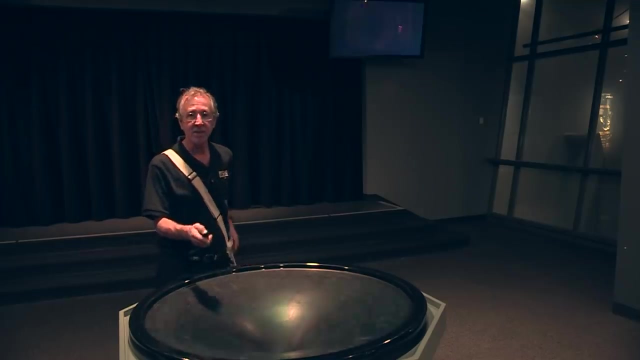 a planet going around the sun. What happens up on the screen is the reality. That's what you see in space. What happens over here is sort of like the behind the scenes, like in the Wizard of Oz. this is like behind the curtains. This is not what you would see if you were to look into space. That's the only thing that you see is the motions. So let me show you a couple ways to do that. Here is the first way. First of all, I need a star. 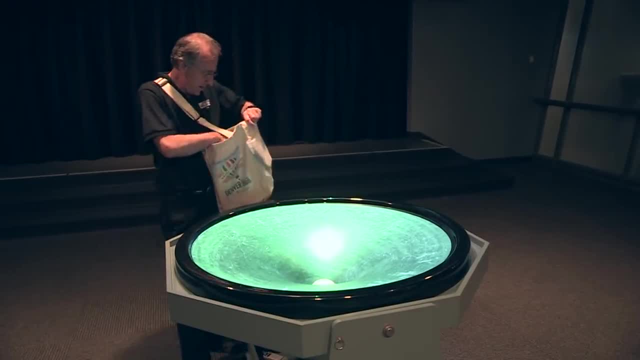 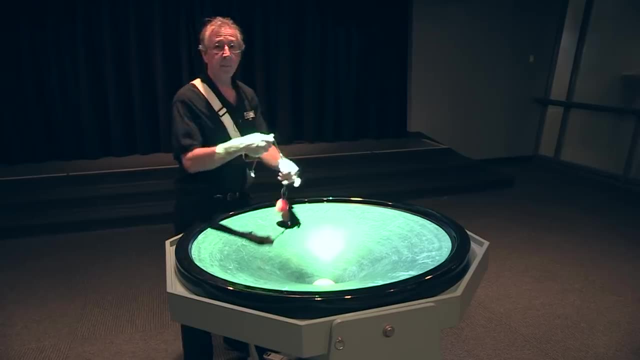 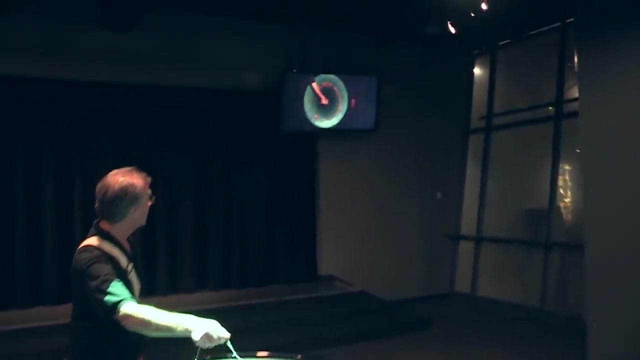 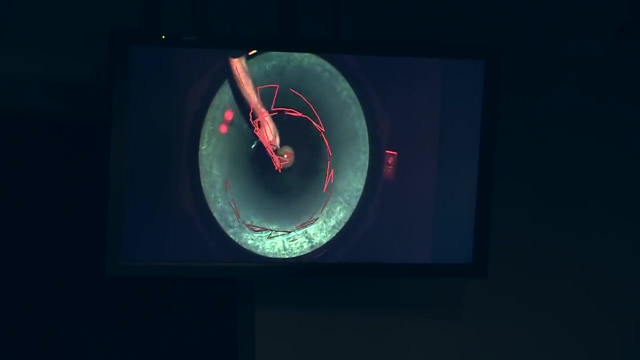 Star goes in there. And here was Sir Isaac Newton's way of making a planet go around the star Ball on a string swinging round and round. If you look up at the screen you can see that it looks just like a planet going around a star, And the reason is because I've got this string over here. They're connected. That's what Isaac Newton did. 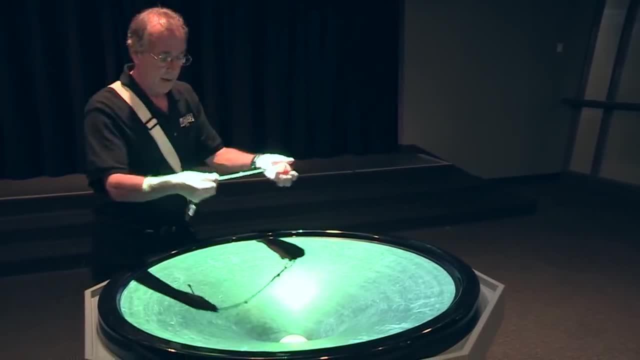 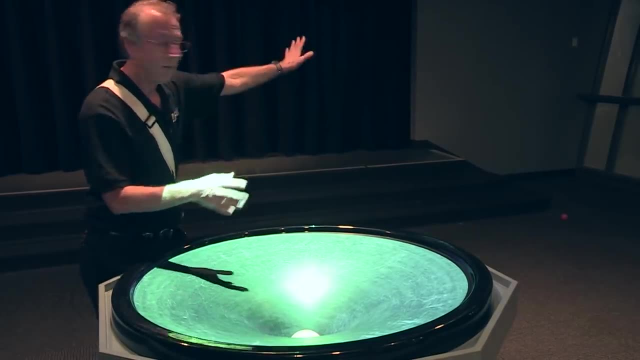 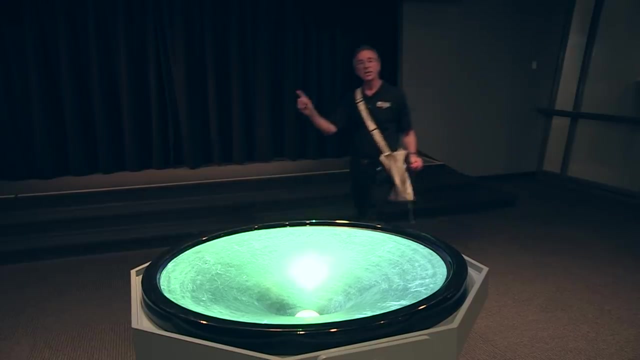 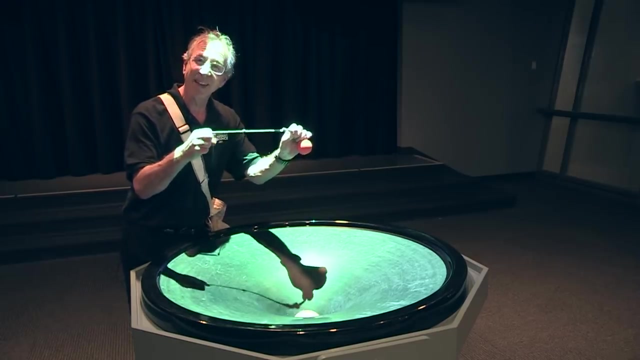 That's what Isaac Newton called gravity. Why did he say that? Because watch what happens if I let go of the string. Sort of flies off into space. So why is it that the earth does not fly off into space? Why is it that the earth keeps on going around the sun? According to Isaac Newton, it's because of some connection between the star and the planet, which he called gravity. 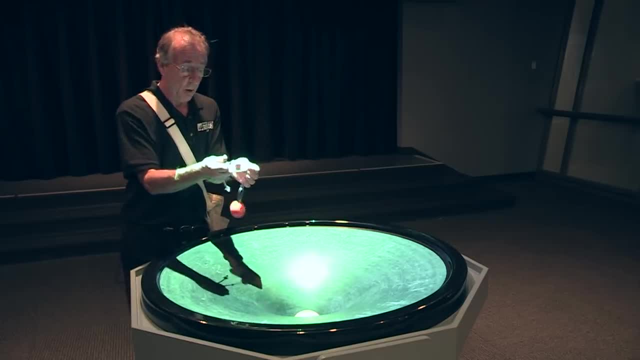 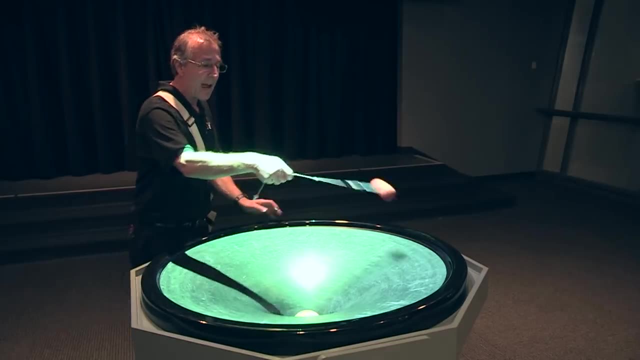 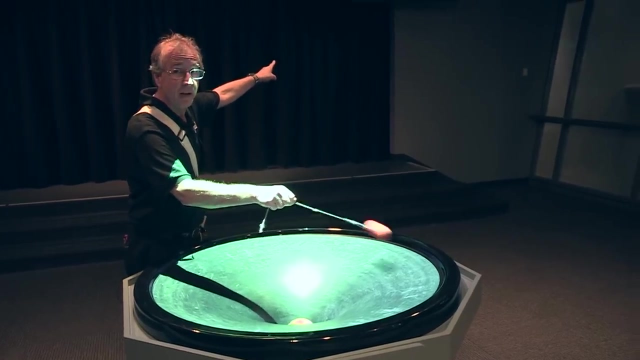 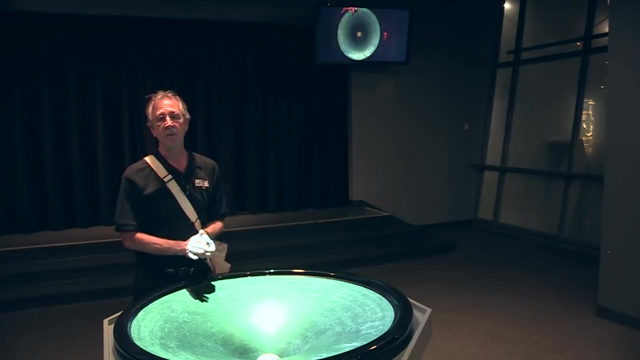 Because you couldn't see that there is no really a rope over there. There's nothing that you can like, feel or smell or see or anything. So he just imagined that there must be some sort of connection, or else how else could you get that if there were no connection? For hundreds of years people looked for that connection, couldn't find it, And then Einstein came along. And Einstein said: you know, the only reality is what's up on that screen. 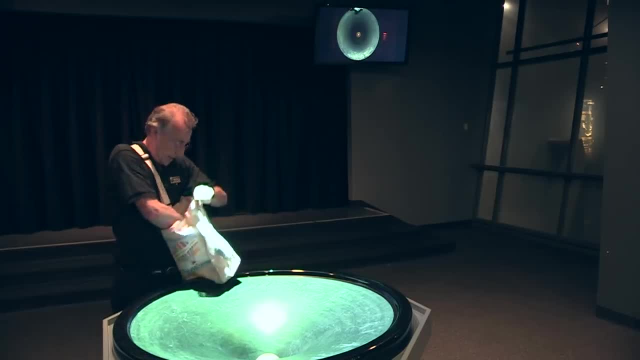 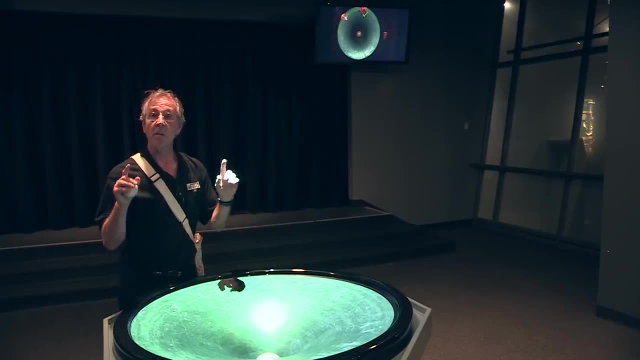 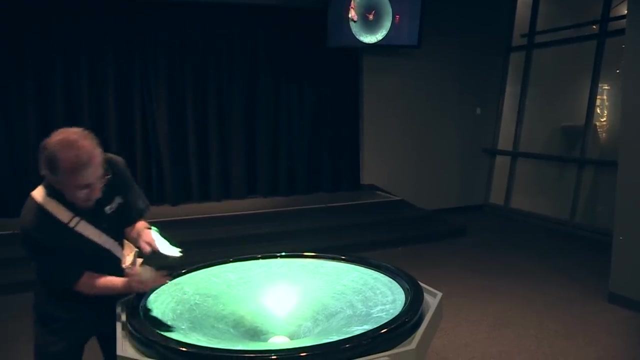 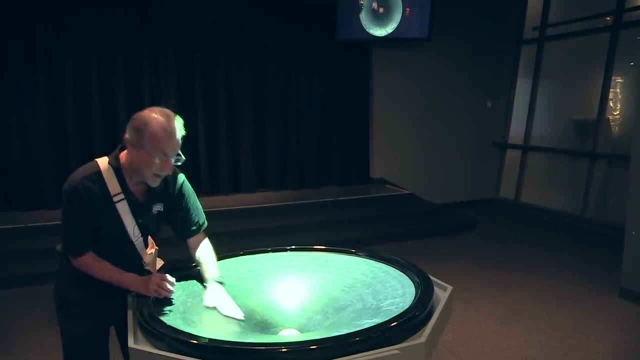 The only reality is a planet going around the star. Is there another way that I can get that same image? So this was his mental way of doing it. He said that there's an extra dimension And you can see it over here, an extra dimension that you don't actually see if you were to look up in the space, And that extra dimension is curved. 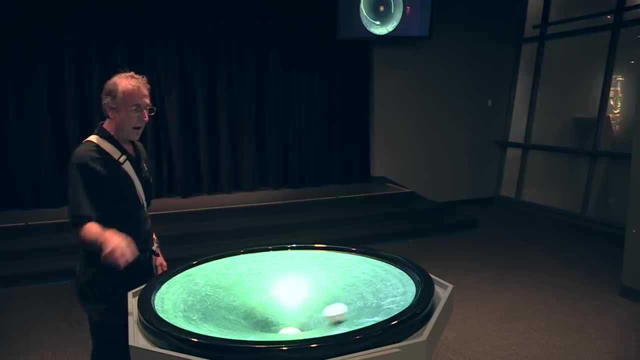 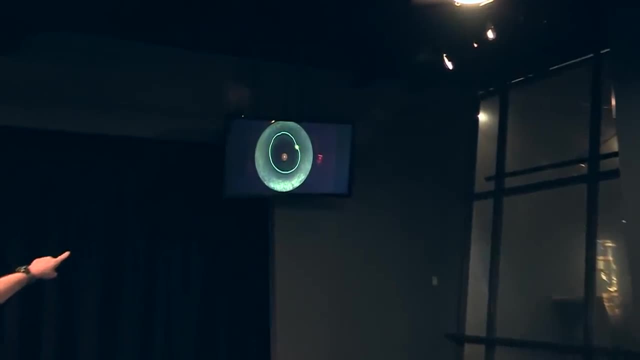 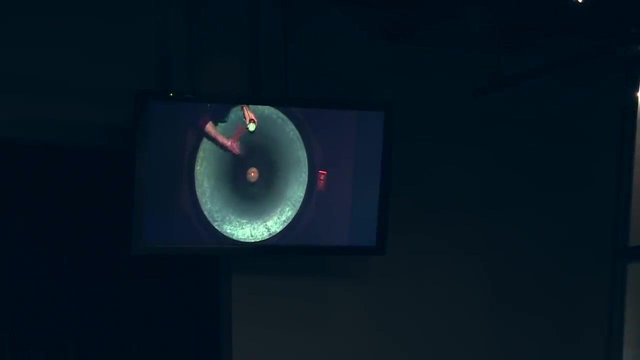 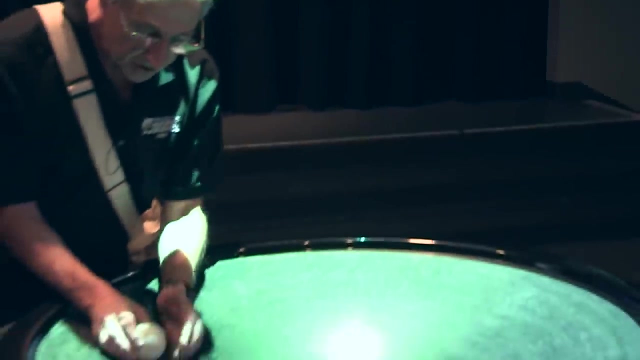 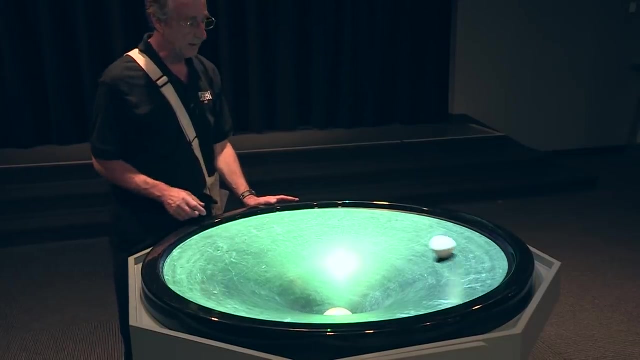 And if I were to roll a ball around that curved space time? if you were to look out in space, up there on the screen it looks like a planet going around a star, But it's not because they're connected with a string. It's because of this curvature over here And, as a matter of fact, the only thing that this ball knows about is the part of the plastic that it actually rolls over, And so it's. 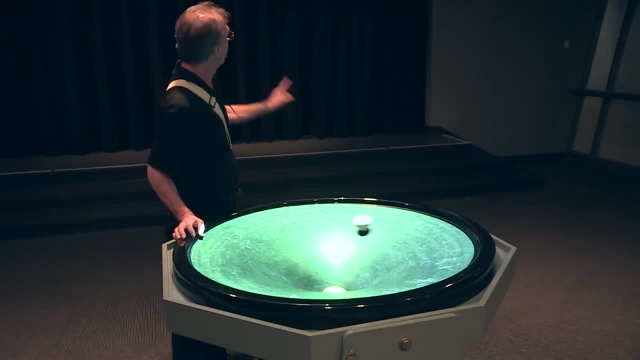 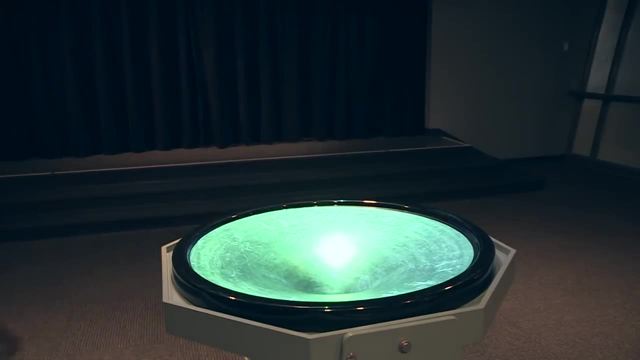 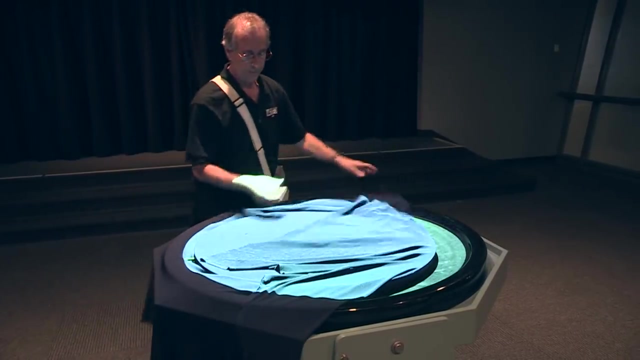 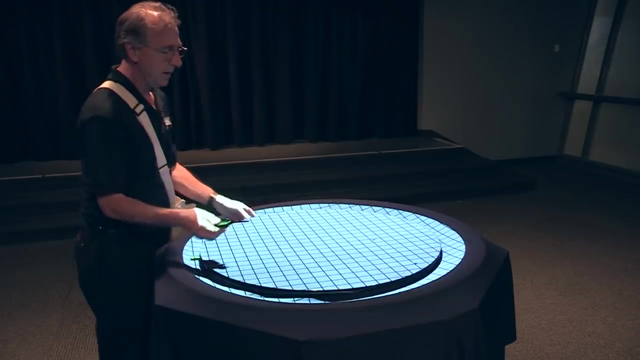 that curvature right where it's rolling over, that causes that. What's more, Einstein said this: I'm going to pull out the fabric of space time And to make it a little bit easier to see, let me put a grid on this fabric of space time. What Einstein said was this: If your 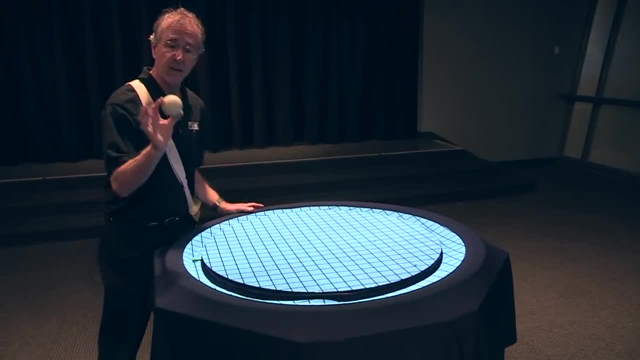 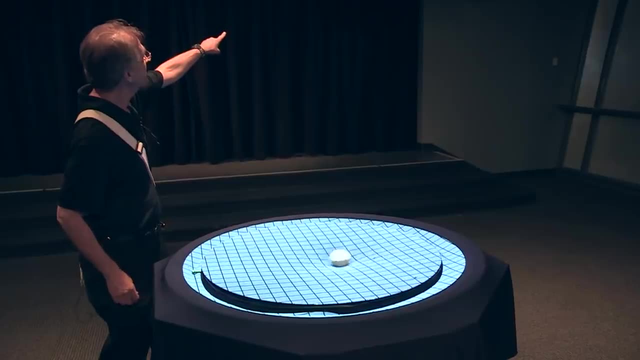 If you don't have anything out in space, that's a flat space. If you were to take a planet, a ball, whatever it is, a rocket ship and roll it, it would make a straight line in that space-time. Watch it up on the screen. 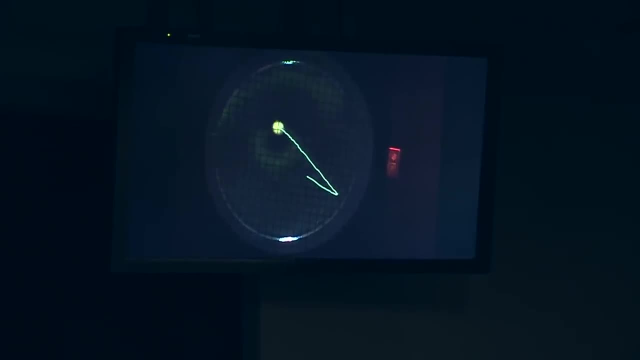 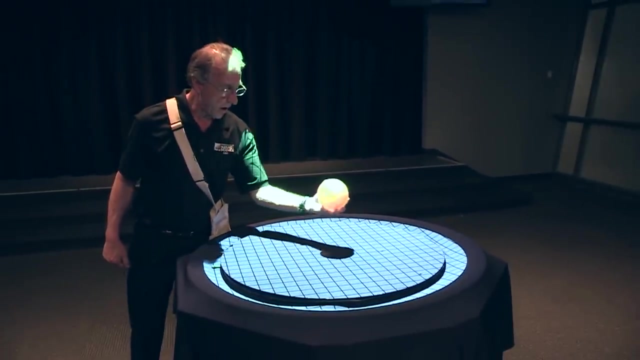 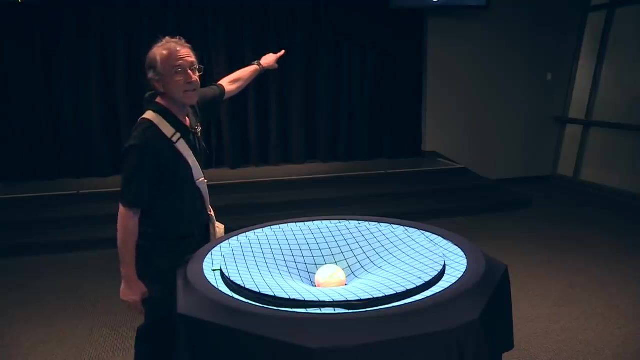 I roll it and it makes a straight line. But according to Einstein, if you go and have a star, that star will bend space-time in that extra dimension that you can't see See. you can't see it bent up over there, but you can see it here. 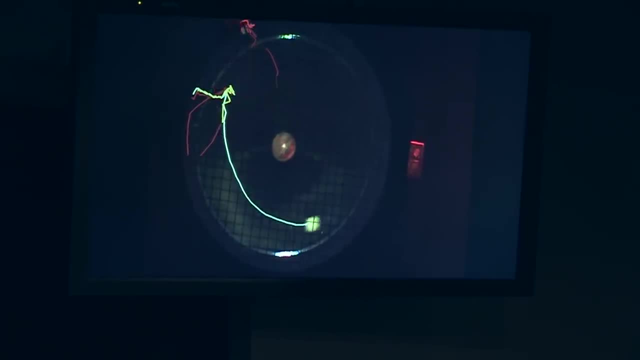 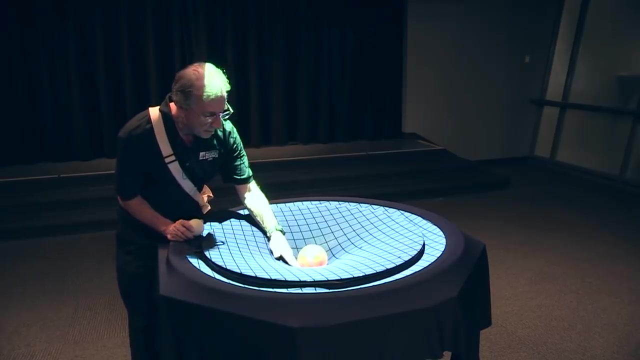 In that bent space-time. if you roll the ball, see now it looks like it's going around and around that planet. So, according to Einstein, there is no connection between the star and the planet. What you have is the star bending the fabric of space, and this little fabric pulls on. 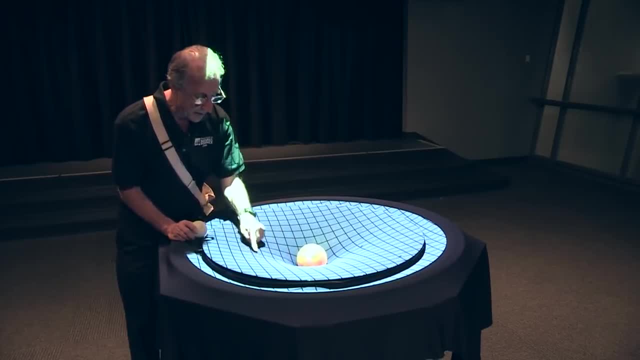 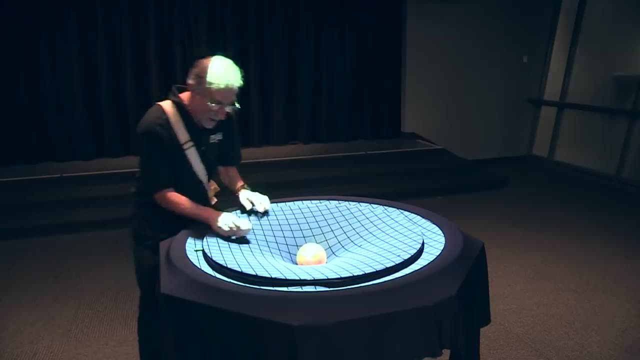 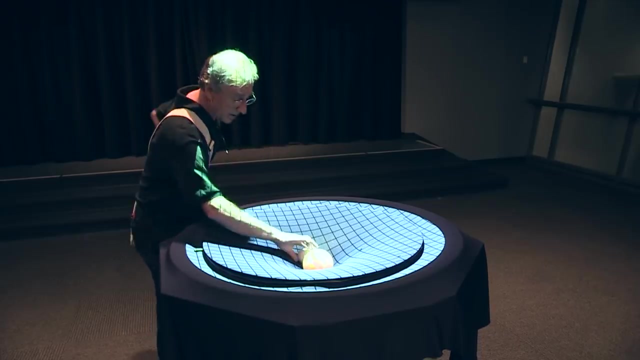 that Which pulls on that which pulls on that which pulls on that. There is no action at a distance, There is only this pulling on the stuff right next to it. And then when the ball goes around and around, it's because of that curvature going around. 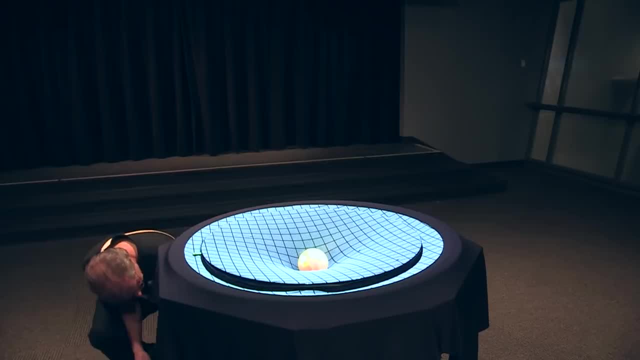 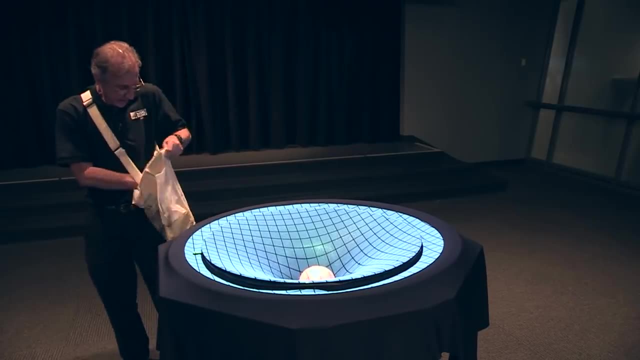 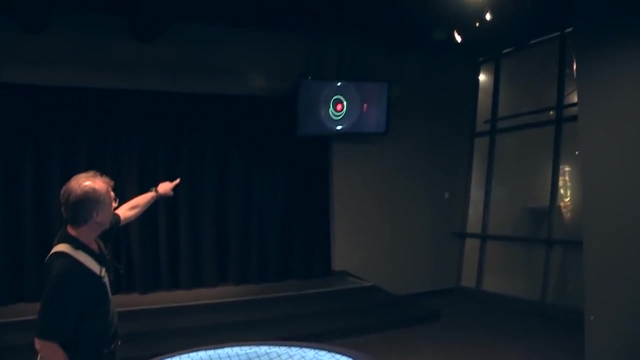 Here's: another thing he said was that if you have a heavier star, a more massive star, and put it in, it's going to curve space-time even more. So watch this. It really looks like a planet going around a star, but once again, it's not because there. 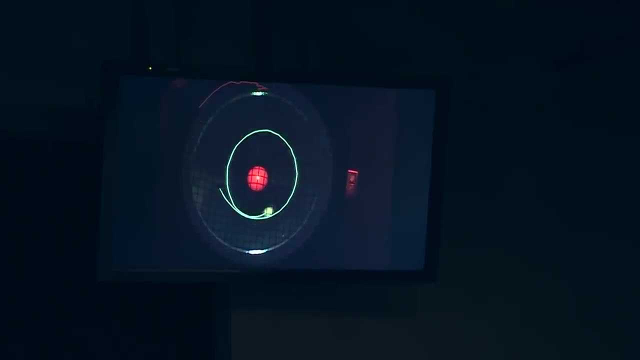 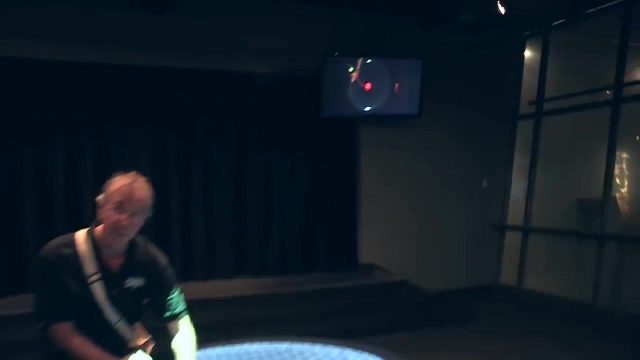 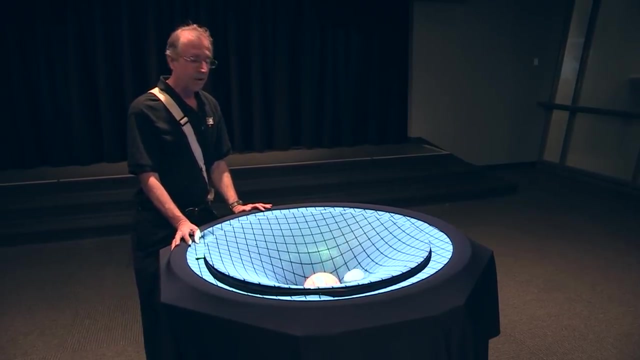 is any connection. It's because there is an extra dimension that you can't see out in space. The star curves that extra dimension of space-time and that curved space-time is what causes it to go around. This is Einstein's general theory of relativity. 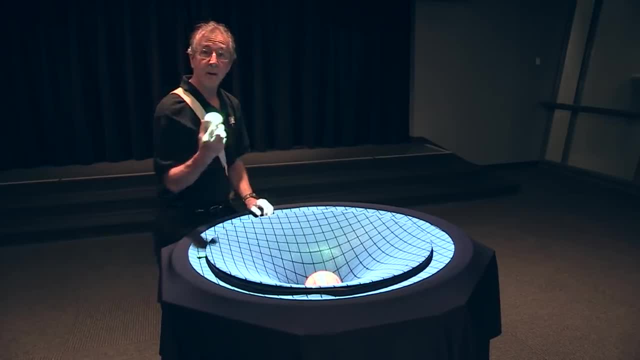 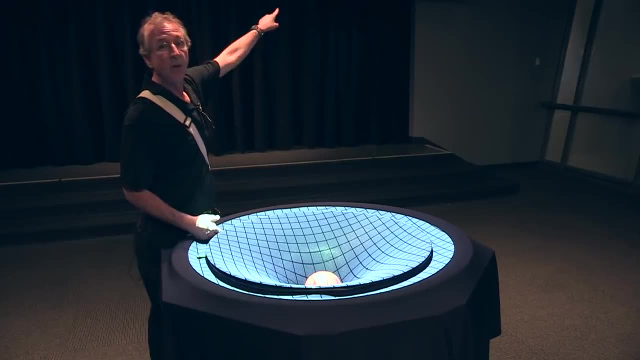 And it is how he explained it- why planets go around stars. So the points that you want to get across are the only reality, is what you see up on the screen, And that's what you keep on directing the visitor's attention to. 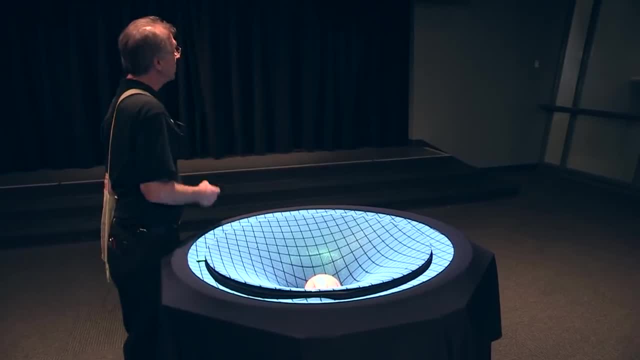 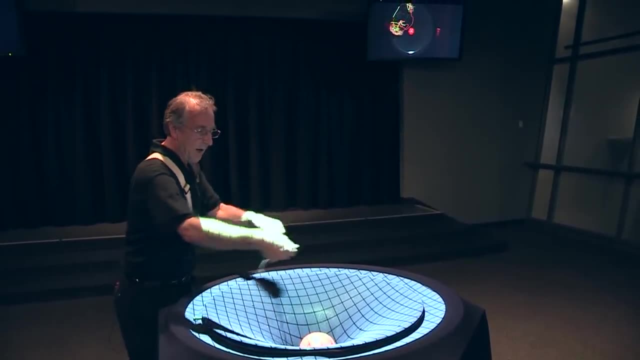 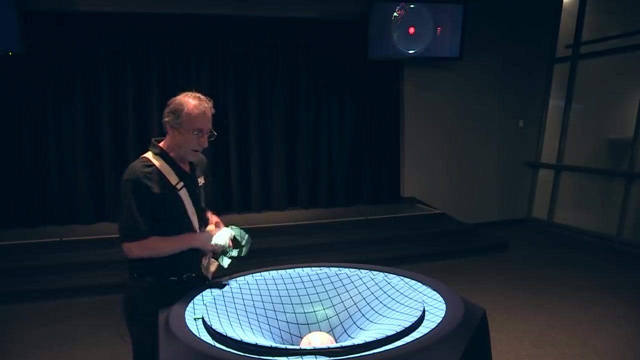 There are two ways to create that image. One way to create that image is using Newton's method of a string connecting the planet and the star, But there were problems with that Einstein's method, which is the star warps spacetime, and that warps spacetime is what